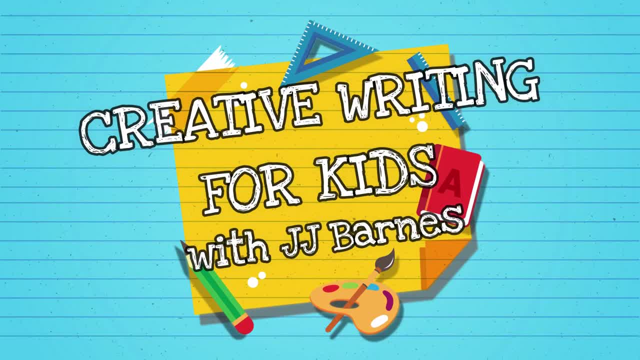 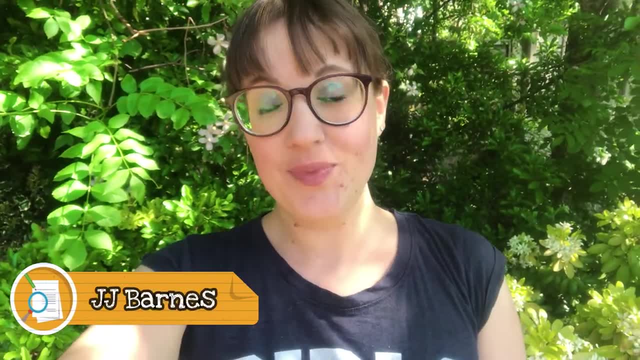 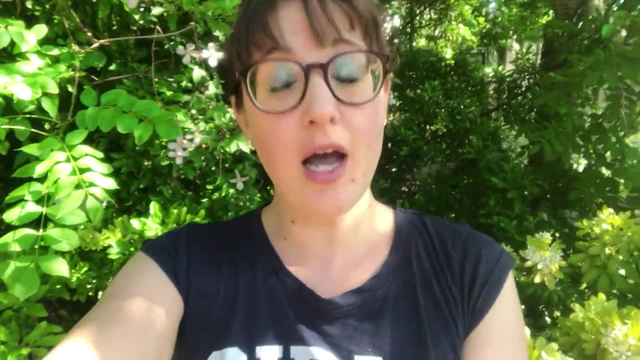 Hi, I'm JJ Barnes and you're watching another episode of Creative Writing for Kids. So today I'm going to be giving you another story prompt and if you have missed the previous story prompt videos, I'll let you know what they are and how to use them first. So a story prompt is when you get. 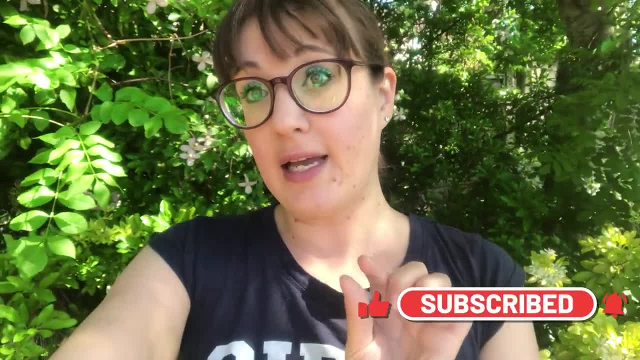 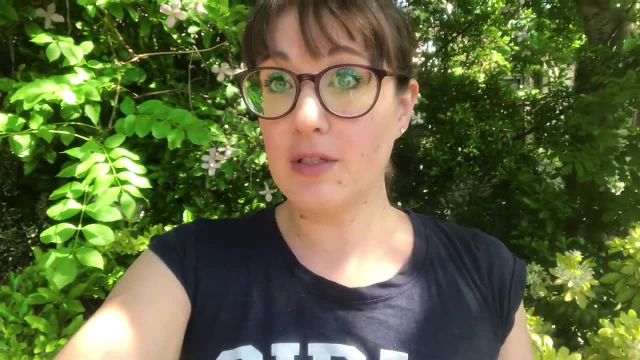 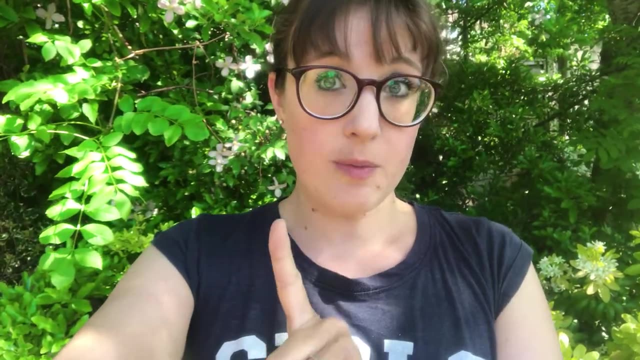 given an idea, a basic, small idea to start your story, and then from that idea you can grow it and you can develop it in any direction you want. but it just comes from a tiny nugget and what you find is, if you give a hundred people one little story prompt, you get a hundred different stories. 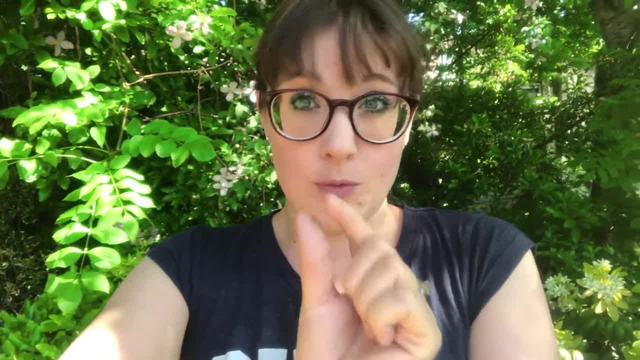 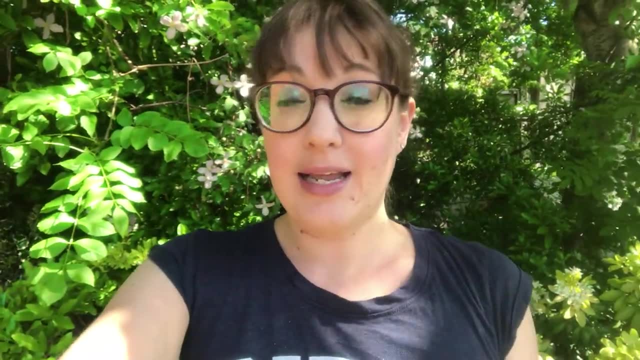 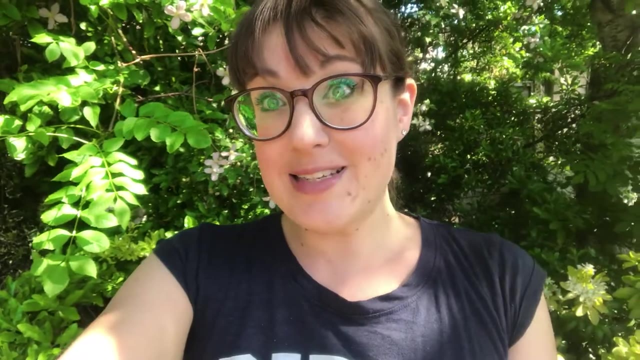 at the end of it, because one little idea, one tiny starting point can grow and grow and grow, and your imagination is what makes it happen and it grows in any direction you want. So it's really fun to see what can happen, because for you it might be obvious. it's. 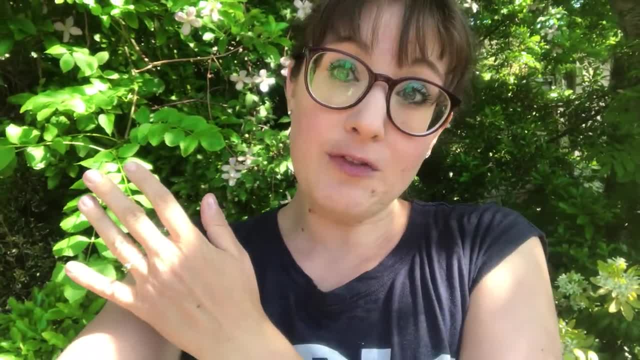 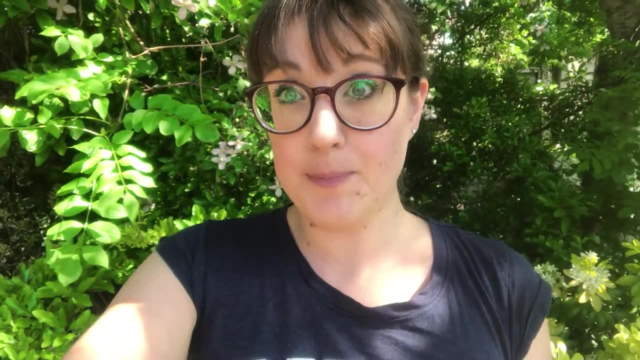 going to go in one direction, but for somebody else it's going to go in a different direction, and then you get to see what other people's ideas are like and what other people see when you see a story idea or how they see it differently. So it's a fun way of looking. 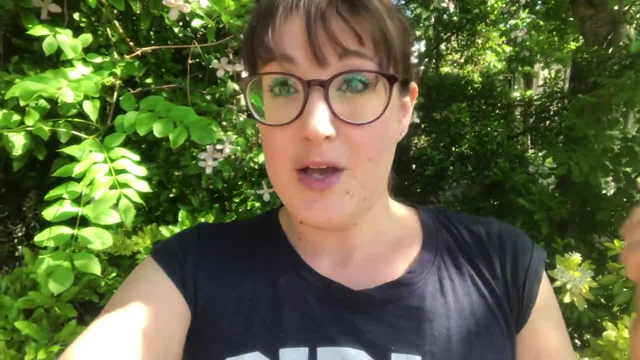 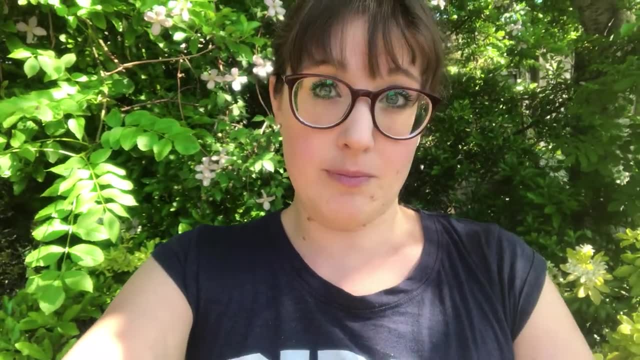 at how other people's minds work. and it's also a great way of getting that first start to your story, because sometimes it's hard to think about what to do to start. So you get your story prompt and then you have it and you grow it. So that's why we use story prompts. The story 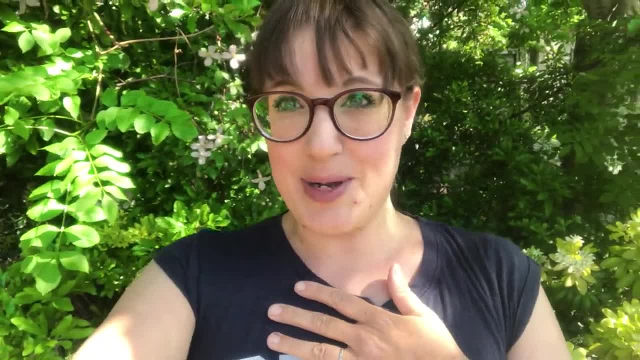 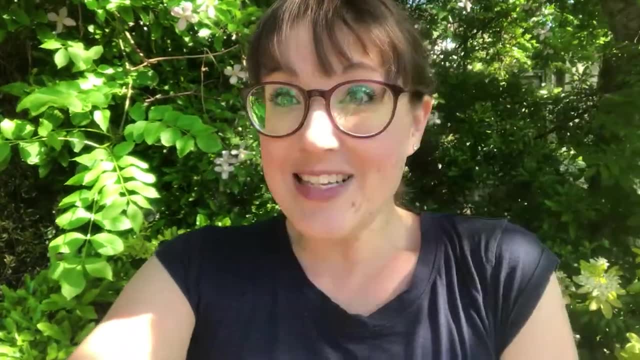 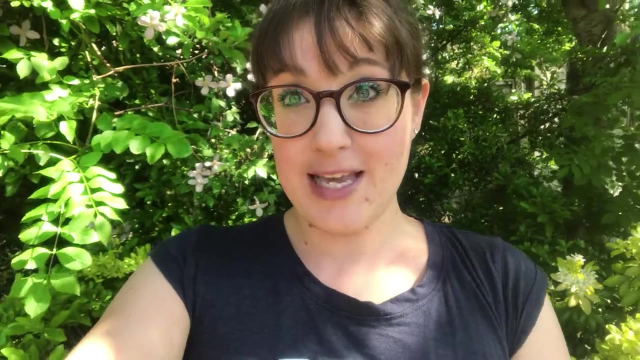 prompt I'm going to give you today is actually one I'm very excited about. Your story prompt is you draw a picture and it comes to life. Now, the reason I'm so excited to do this story prompt with you is because I'm actually going to share on the Creative Writing for Kids page on Facebook how I 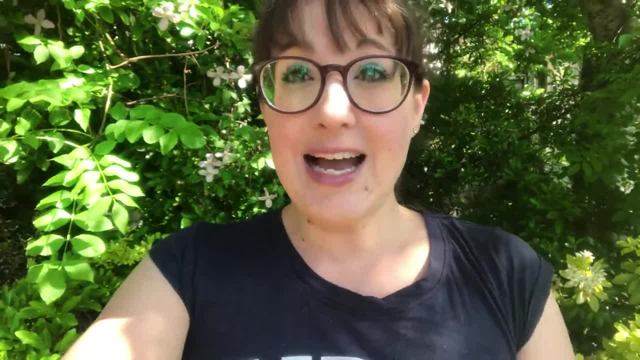 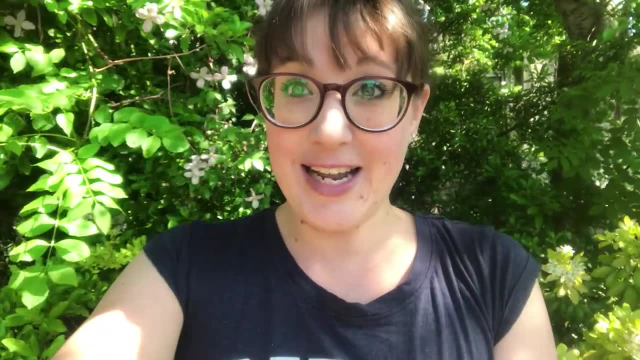 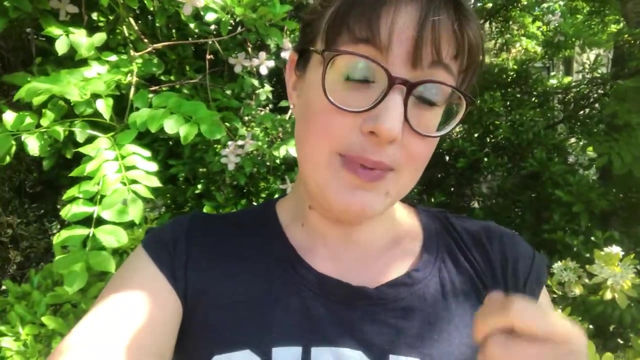 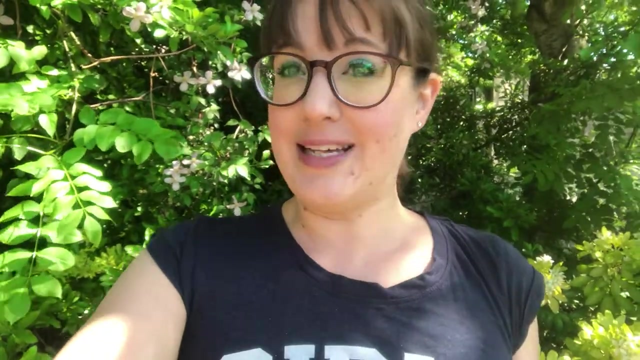 wrote from that story prompt because actually that was the first idea I had when I wrote Lily Prospero and the Magic Rabbit. That was the story prompt I got to write for my book. So I'm going to share with you what I did with that and I'm going to post it. I might post either a whole chapter or 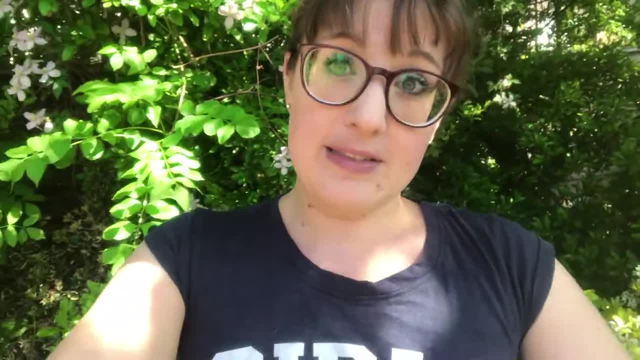 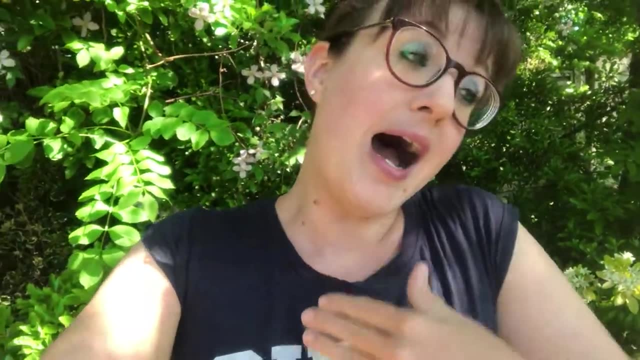 a few pages, but I'll pick a section where that happens in the book and I'll post it because then you can read it, you can look at it and you can see how my mind went with that, where I went, how I grew that story. So I'm going to share with you what I did with that and I'm going to post it. 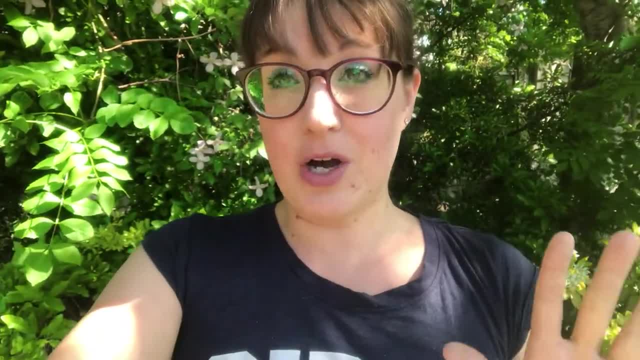 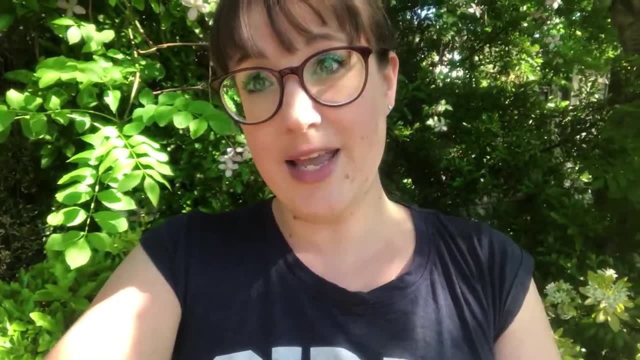 that little nugget, that little story idea, into a whole story and that should really help because you'll be able to see what I'm talking about. then You'll be able to really fix in on what the story is and how I grew from that little prompt and I really hope that you'll be interested as well. and 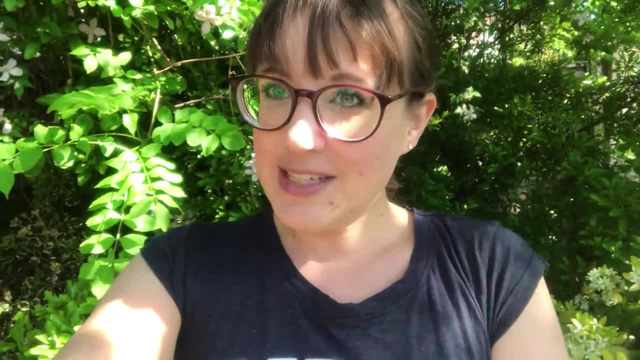 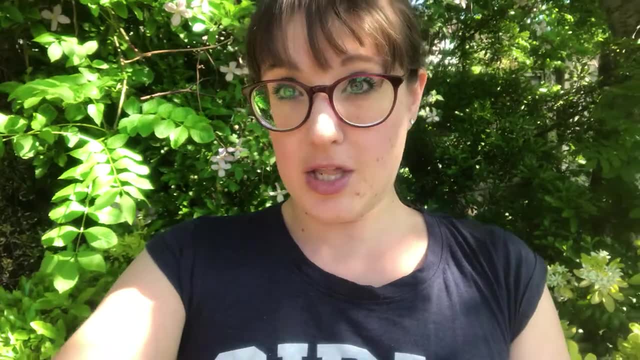 enjoy what I wrote. So, yeah, that's my video today: a story prompt that you are going to use and you're going to try and think about where it's going to go. So I'll talk you through how you're going to think about it now. So you draw a picture. 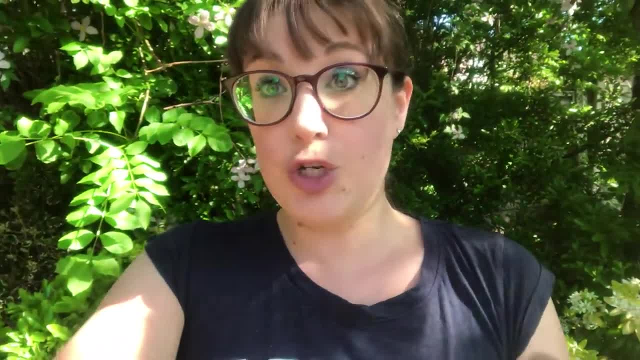 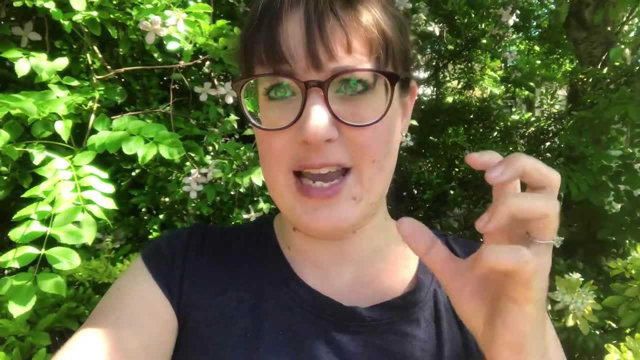 what do you draw? Did you draw something good, Something bad? Did you draw a scary animal? Did you draw an alien? Did you draw something pretty and delicate, like a butterfly or a scary shark? Right, so you have to decide what it is you drew that's going to come to life, and then you have to 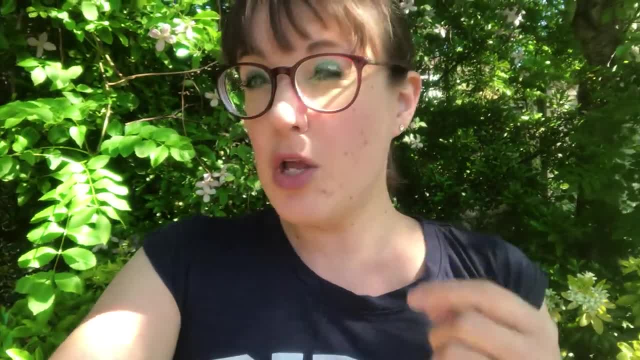 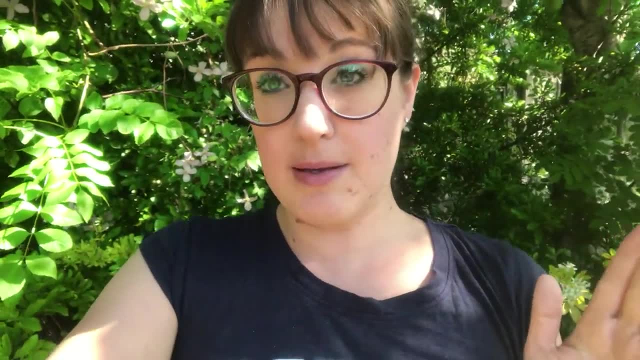 work out. did you know it was going to come to life? Did you know you have something magical in your pen or your paper or your pencils or your paint? or is it something that's inside of you that made it come to life? So did you know it was going to happen or not? 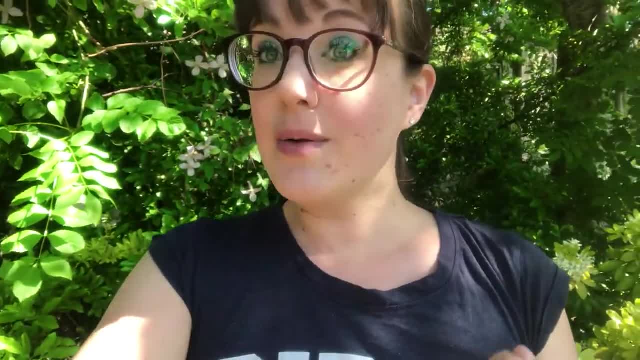 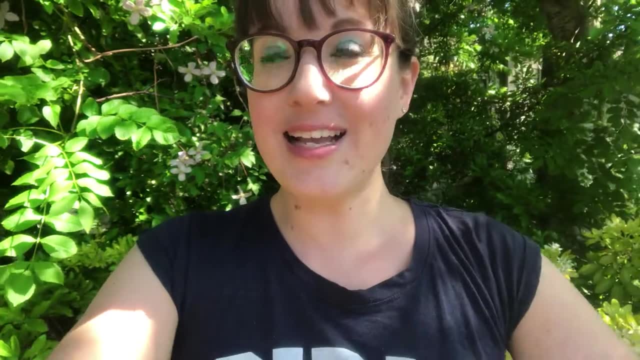 Are you happy that it's happened? Are you scared? Are you excited? Is it something you've been trying to do? and you've been trying to work a spell, and when it happens it's: yes, that is what I've been trying to get to happen. it worked, hooray, Or is it? oh no, I didn't want this to. 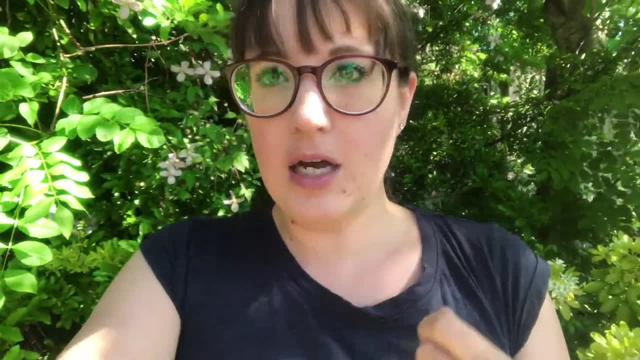 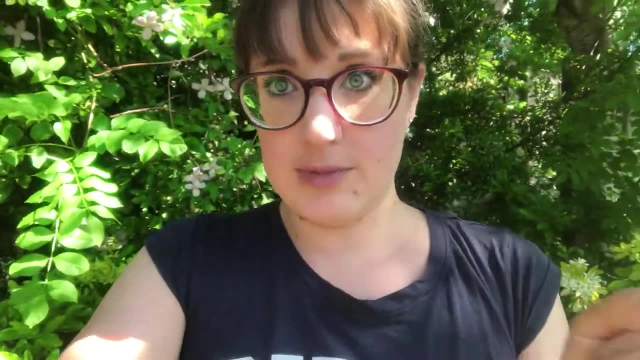 happen. this is a disaster. Where are you when it happens? Are you at home, in your bedroom? Are you at school? Are you at art club? and everybody else's drawings are staying normal, but yours has come to life. Do you have to hide the fact it's come to life, or can you? 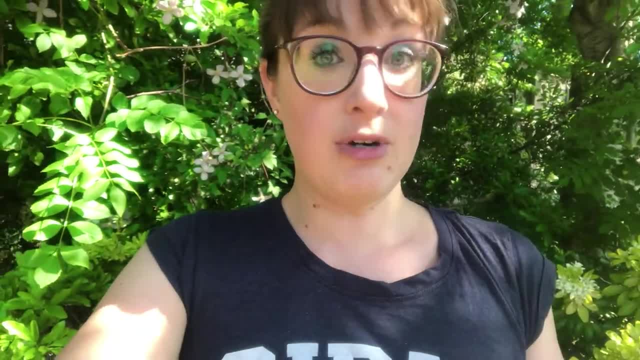 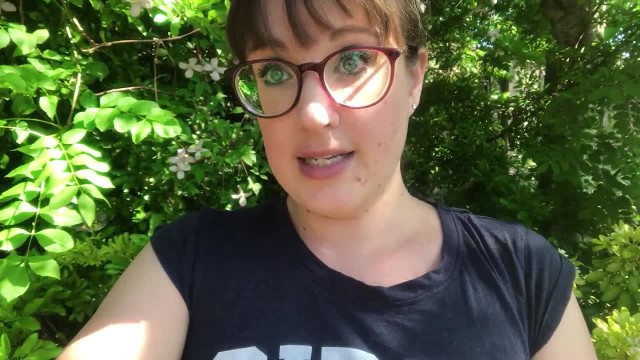 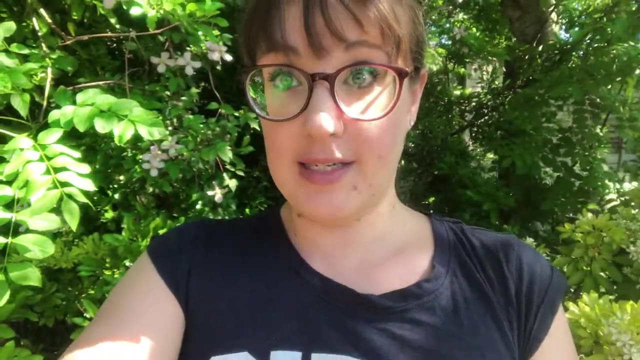 celebrate it? and then who do you tell if it's a surprise? do you have anyone you can trust to tell that that has happened? does this make sense? you look at the story idea and you ask questions. you grow up from the story by asking questions to yourself about how you're going to react to it coming to life and